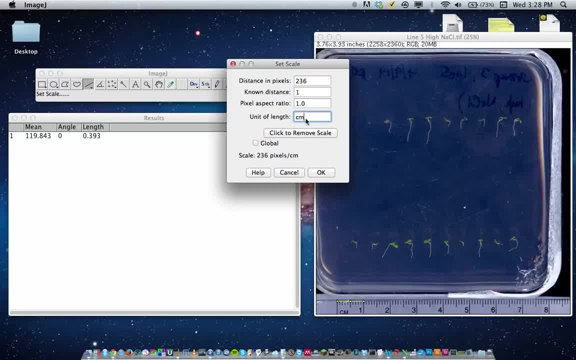 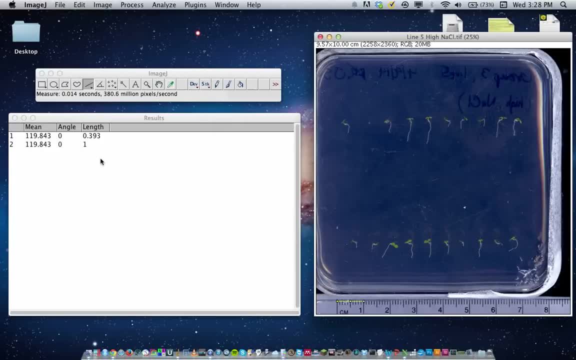 Leave the pixel aspect ratio, change this to centimeter and hit OK. Now, if I hit Command-M again, we should have a length of 1 centimeter, So that's good. So now, if I wanted to measure the length of this root or a hypocotyl, I would recommend. 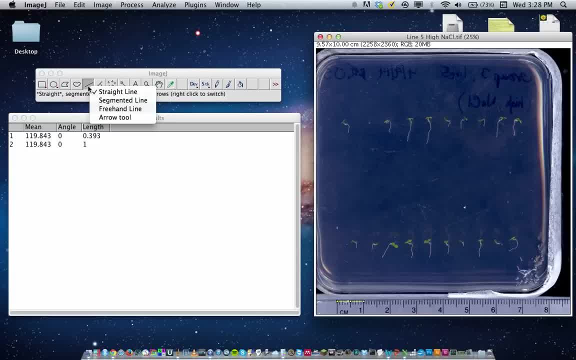 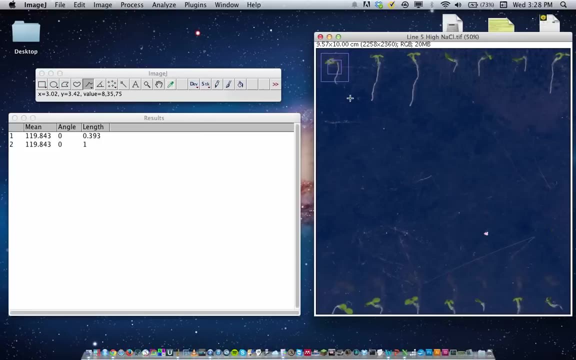 using the freehand tool. So you can go to the straight line segment, right click, use the freehand line tool and you can also zoom in the image to make it a little easier to work with. So if I want to measure the length of this root or pretend it's a hypocotyl, I can. 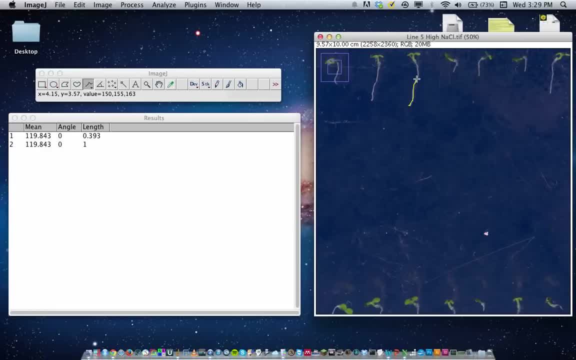 just click and drag the line over the length of the root, hit Command or Control-M, and it'll give us the length. So that's for one root. here's another root: Command-M. yadda, yadda easy. 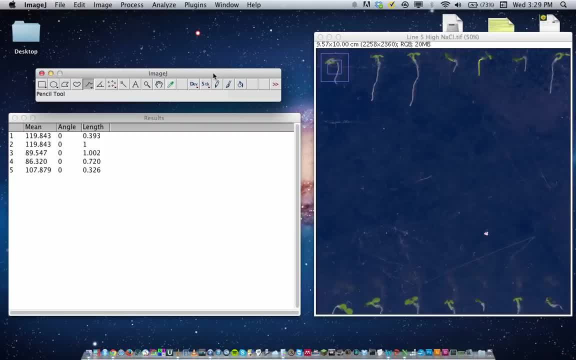 OK, and for next week you'll be checking the angle of growth for the Gravitropism and Phototropic mutants. So to do that you use this angle tool next to the freehand tool. So if I wanted to test the angle of this root and shoot angle, click first at one end of 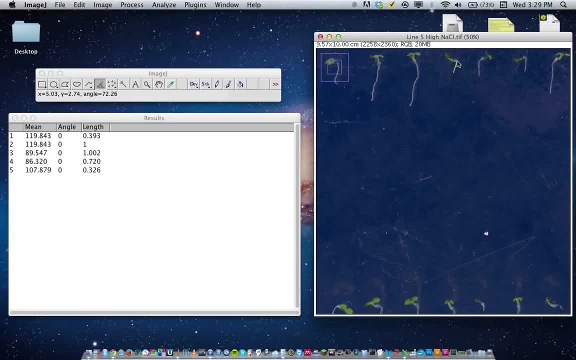 the thing: click first, click again where you want the point of the angle to be, and then click one third time, and you should have some kind of angle here and if you hit Command or Control-M, it'll actually give you what the angle is. 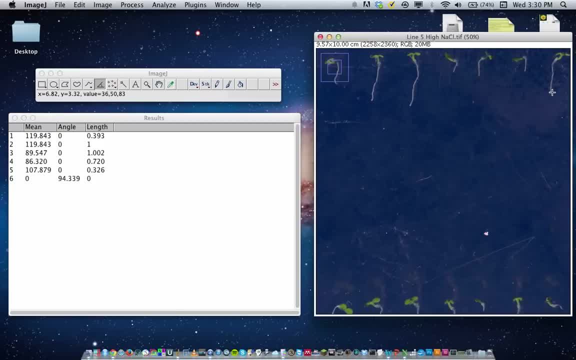 So another example, if I want to try here: Control-Command-M, and we're given the angles, So basically to use this, click once, click again, click third time, Command-M, and that's all she wrote. Good luck, let me know if you have any questions. sayonara.